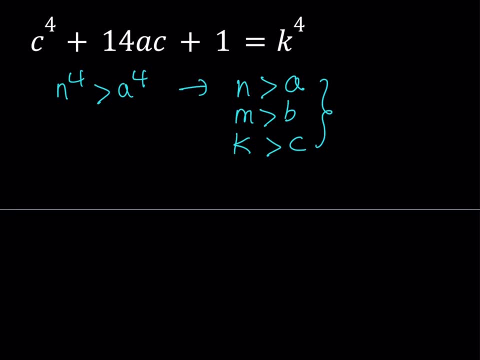 than a, and n and a are both positive integers. we can say that obviously the smallest value for n would be a plus one, So n needs to be a plus one or larger. So I can write these inequalities in a less strict way, such as: n is greater than or equal to a plus one, m is greater or equal to. 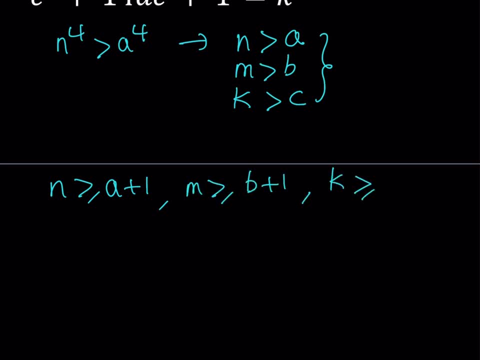 b plus one and k is greater than or equal to c plus one. Awesome. Now, this is helpful because if we're going to write these inequalities in a less strict way, we're going to have to, because if you raise both sides to the fourth power, you're going to get the following: So if 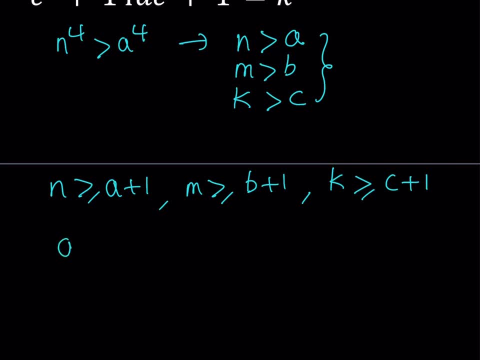 you look at our first equation, it was a to the fourth plus 14ab plus one is equal to n to the fourth, And now we know that n is greater or equal to a plus one. Therefore, n to the fourth power is going to be greater than or equal to a plus one to the fourth power, And we can do the. 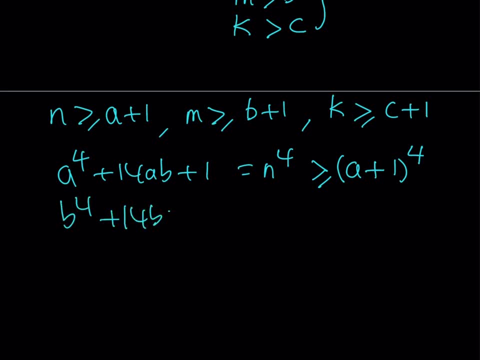 same thing for the second equation: b to the fourth plus 14bc plus one. So we're going to raise both sides to the fourth power, because these are all positive quantities and we can do the opposite. And same thing works for c to the fourth plus 14ac plus one, which is equal to k to 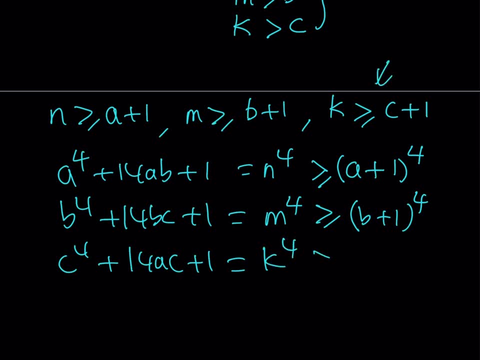 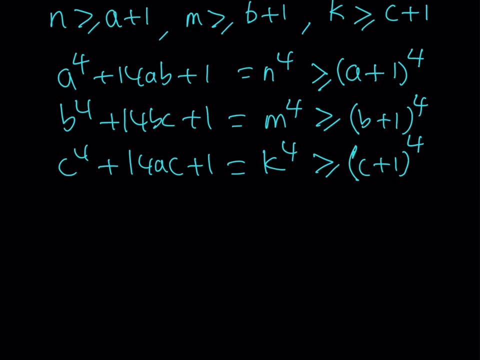 the fourth, but k is greater or equal to c plus one, as you can see here. Therefore, k to the fourth power is just going to be greater than or equal to c plus one to the fourth power. So we kind of get this nice set of inequalities And forgetting about these terms here. 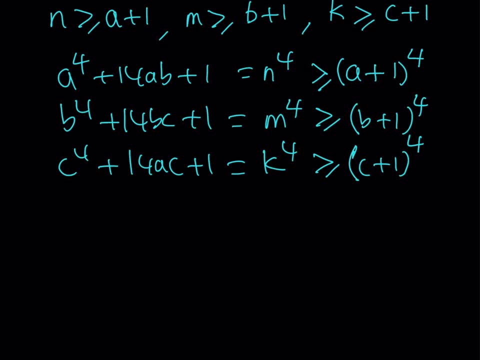 you know, the ones that are in the middle, kind of like. forget about these ones. we can safely associate the first one and the last one, So let's go ahead and see what happens, Taking the first one into consideration, a to the fourth plus 14ab plus one is greater or equal to. Now I'm going to 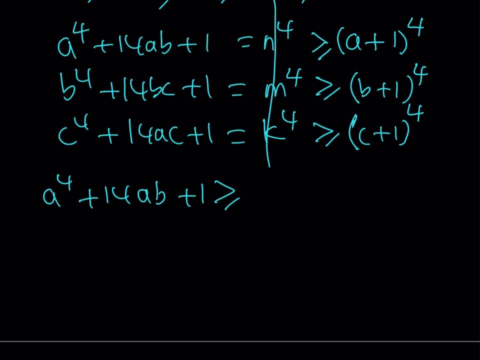 expand the right-hand side. I have a plus one to the fourth power, The right-hand side. let's go ahead and expand it. It gives us a to the fourth power plus 4a, cubed plus 6a, squared plus 4a plus one. So some of these terms are going to cancel out. Let's go ahead and. 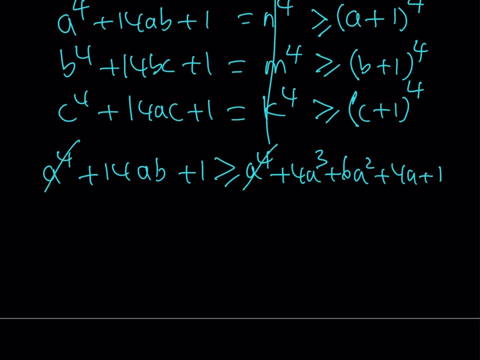 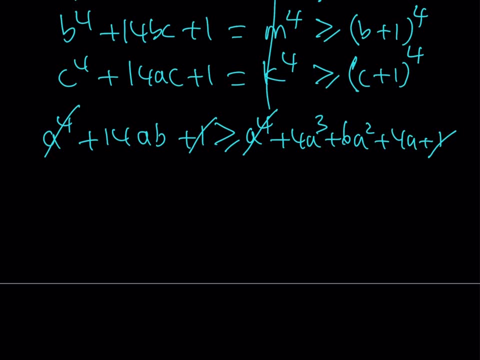 simplify this: a to the fourth is going to cancel out, One is going to cancel out, And obviously we can divide both sides by two now and we get the similar, or I should say: well, let me do the following, Let me rewrite this inequality: after the cleanup: 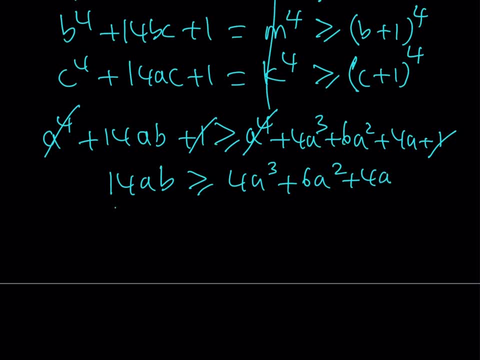 And then I'll tell you what we're going to do next. Obviously, we can just go ahead and factor out a 2a here And that's going to give me 2a squared plus 3a plus two, And whatever I do, 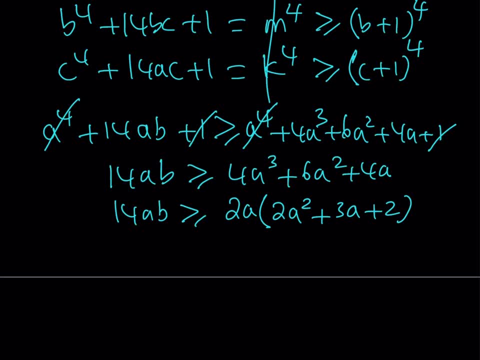 with the first equation, or inequality. I'm going to be doing it for all of them, So I don't really need to go through all the steps here. Let me just show you one Now. we can divide both sides by 2a. 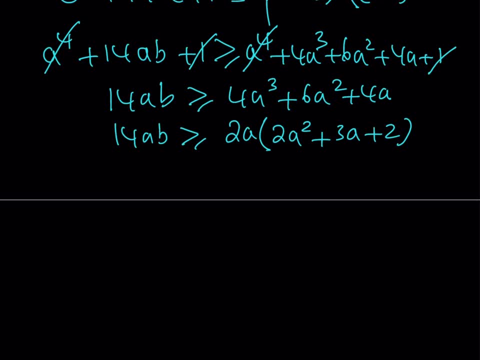 Notice that a is not zero, It's a positive integer. If we divide both sides by 2a, you get, oh man, 2a, 2b or not 2b. Anyways, we missed that one. 7b is going to be greater than or equal to. 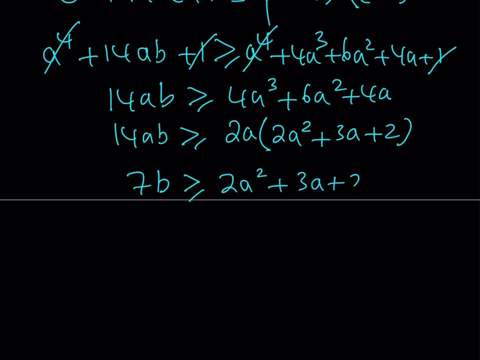 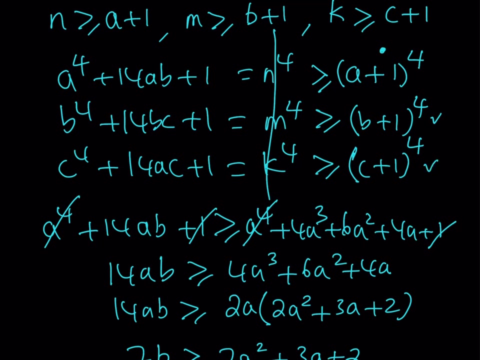 2a squared plus 3a plus two, And similarly, whatever we did for the first equation, we can do for the second equation And basically what we did was expand the right-hand side and then simplify as much as we can, and then factor and then simplify. And the third one. 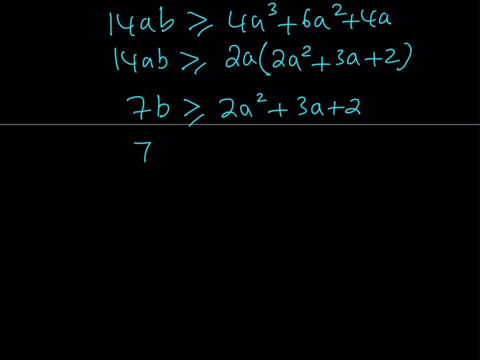 So second and third one is going to give us something similar to this. it's going to look like 7c is greater or equal to 2b, squared or not- 2b plus 3b plus two. And then, with the 7a, we're going to get greater or equal to 2c squared plus 3c plus two. Great, So after. 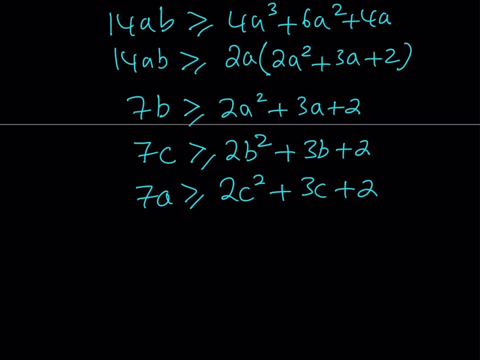 all these manipulations, we are getting these inequalities, which is kind of nice, But it's still not very nice, so we have to make it nicer. How do you make it nicer? We can add these inequalities. Let's go ahead and add them up. 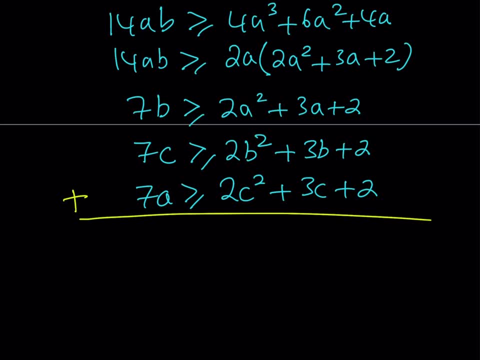 And obviously when you do, some of the terms are going to simplify, you know we'll bring them together, so on and so forth. So we get 7a plus 7b plus 7c is greater or equal to two times a squared, b squared, c squared. but well, I don't need to factor it. 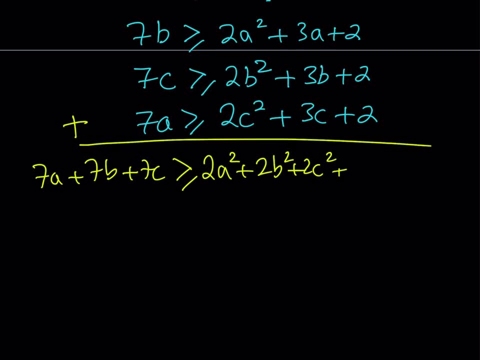 because I need them separate And then 3a, 3b, 3c and then plus six, right, Okay? Now what we can do here is significant. We can bring the 7a, 7b, 7c to the right-hand side and then kind of switch sides or flip sides, so that we can have 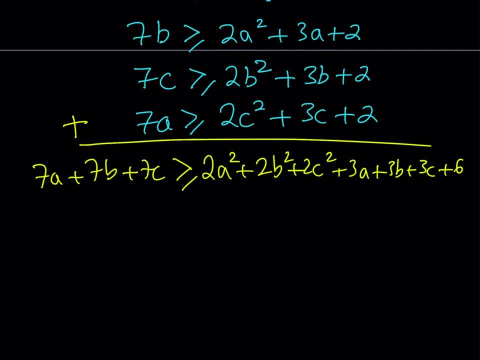 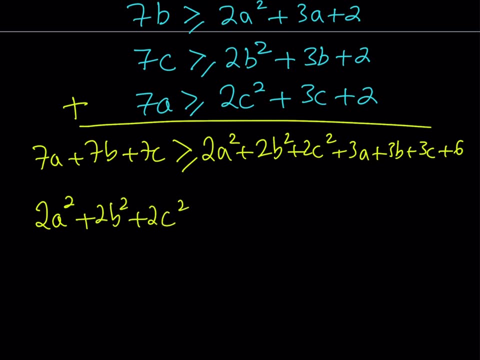 the terms on the right-hand side, So the left-hand side becomes the right-hand side, and vice versa, And this gives us the following: 2a squared plus 2b squared plus 2c squared. Now notice that we're subtracting 7a from 3a. that's going to become negative 4a, negative 4b, negative 4c. Or, if you 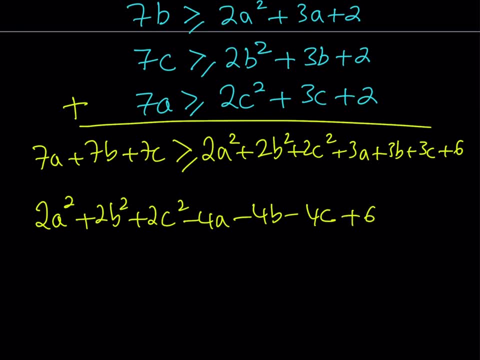 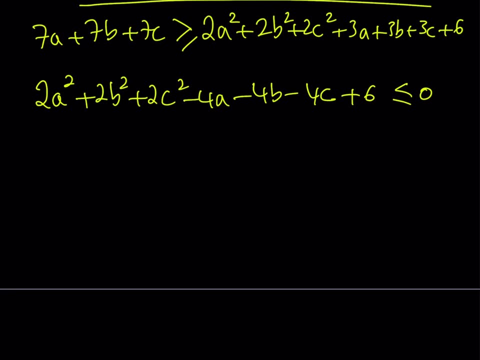 want to call it minus, that's fine too, And plus six is going to be plus six because it is already on the right-hand side. So now we're going to get the terms on the right-hand side, And then we're right- Great. So this expression can be simplified even more. Let's divide both sides by 2. And 2 is 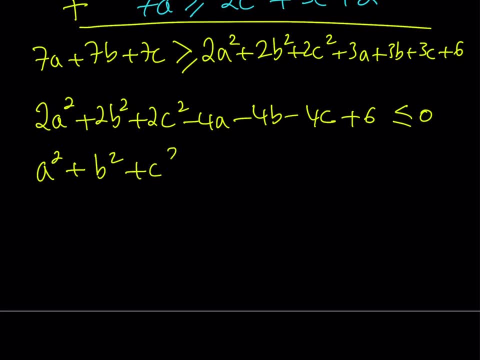 a positive number. so it's cool. a squared plus b squared plus c squared minus 2a, minus 2b, minus 2c plus 3 is less than, or equal to 0.. I know what you're thinking. Oh man, wouldn't that be nice. 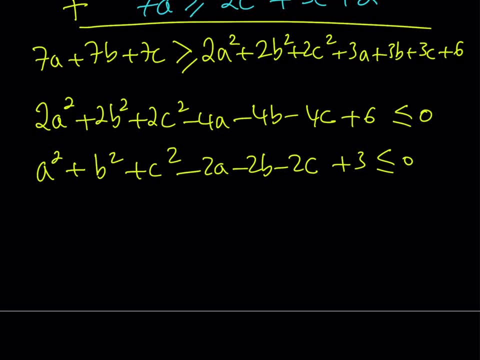 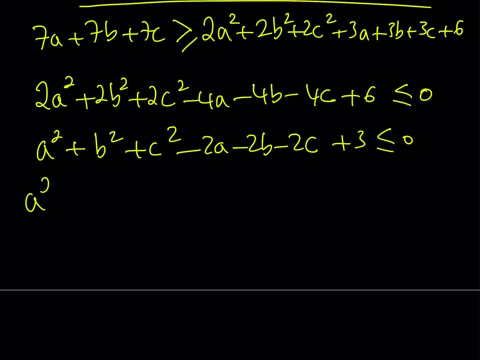 if we had a plus b plus c, quantity squared, or something like that. But don't worry, this can still be simplified. Now we're going to be separating the 3 into 3 pieces and write our expression this way: a squared minus 2a plus 1.. And now we're going to get b squared minus 2b. 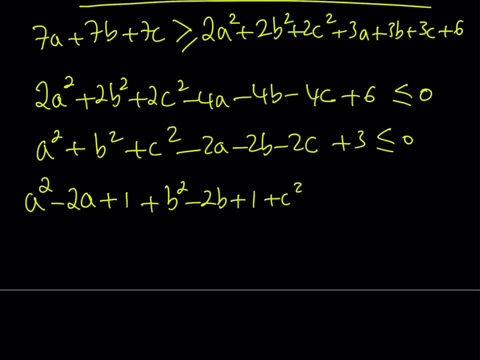 yay, 2b or not, 2b plus 1.. And then c squared minus 2c plus 1.. And 1 plus 1 plus 1 is equal to 3, so it's all good, But guess what? This gives us the sum of 3 squares. Isn't that awesome. 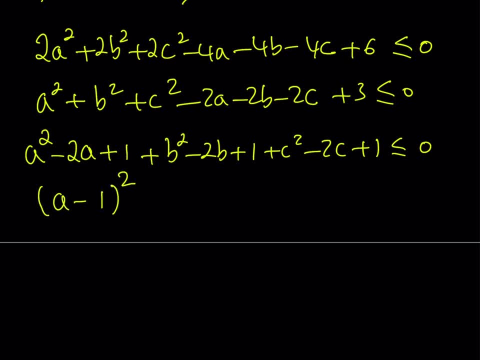 Well, that was intentional, right. When they wrote this problem, obviously they thought about this idea, But it's really cool to come up with something like this. Anyways, so I can write it as a sum of 3 squares and something that is less than or equal to 0.. But 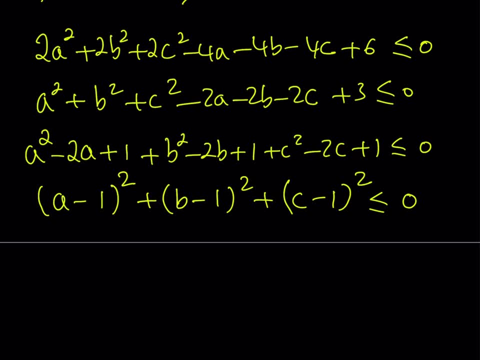 as you know, sum of squares in the real world cannot be negative, so it has to be 0.. This gives us what This needs to be 0,, this needs to be 0, and this needs to be 0.. So from here we get.